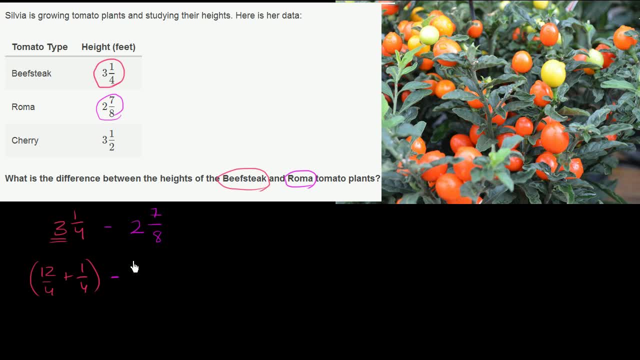 And from that we're going to subtract 2 and 7 eighths. 2 and 7 eighths is the same thing as 2 plus 7 eighths. 2 is the same thing as 16 over 8 plus 7.. 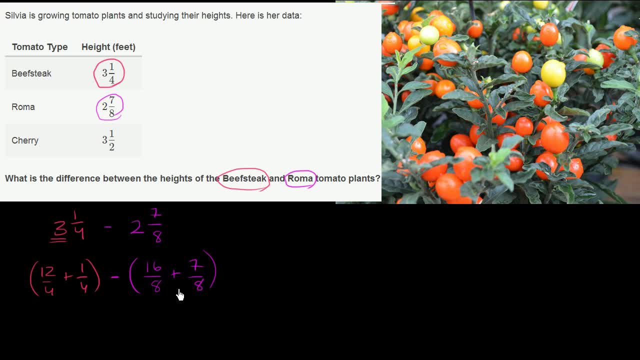 OK, 7 over 8.. So this is essentially what we are trying to figure out. Now, what is 12 fourths plus 1 fourth? It's 13 fourths, 13 over 4.. And then what's 16 eighths plus 7 eighths? 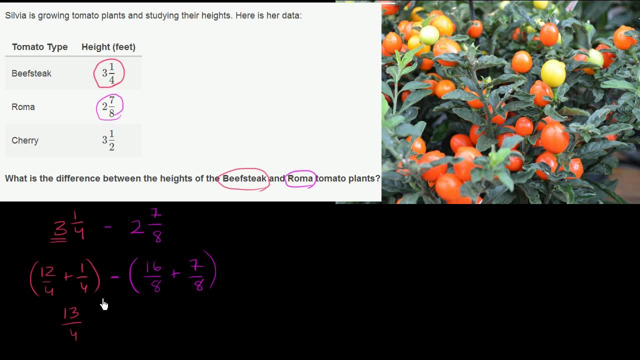 Well, that's 23 over 8.. So this is going to be minus 23 over 8.. Now we're subtracting one fraction from another, but we have different denominators, So we can't make sense of this until we. 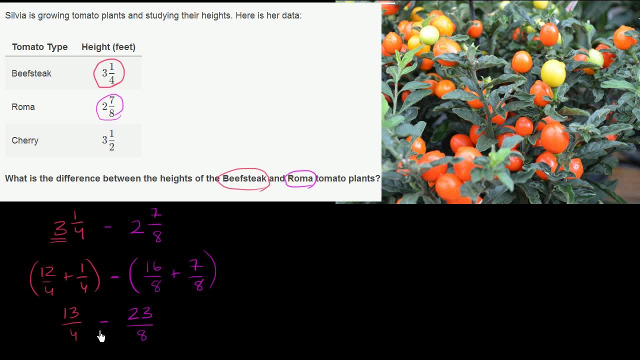 have the same denominator. And so what is the least common multiple of these two denominators of both 4 and 8?? What is the smallest number that is divisible by both 4 and 8?? Well, 8 is divisible by 8, and 8 is also divisible by 4.. 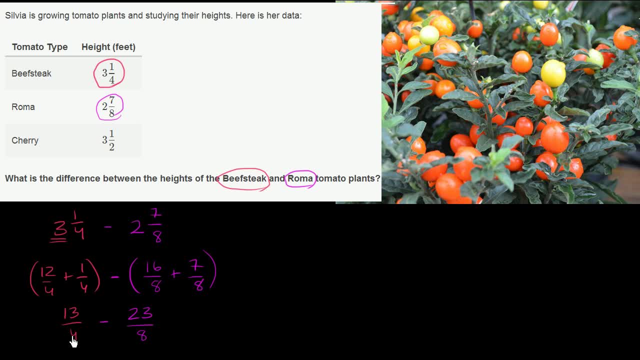 So if we can rewrite 13 over 4 as having 8 as a denominator, then we are all set. So let's try to do that. So we're going to write both of these as 8, with 8 as a denominator. 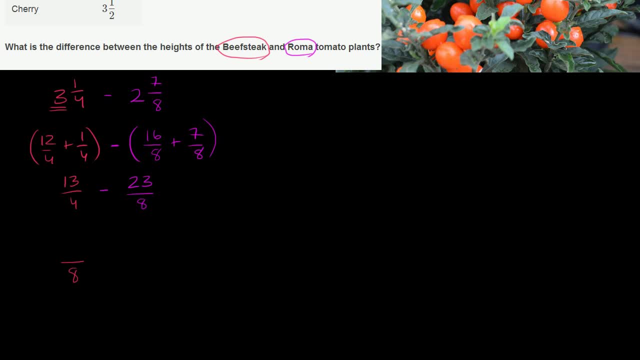 This one already has it. So 13 over 4,. I'm going to have it with 8 as a denominator. So to get from 4 to 8, we have to multiply the denominator by 2.. So in order to not change the value of the fraction, 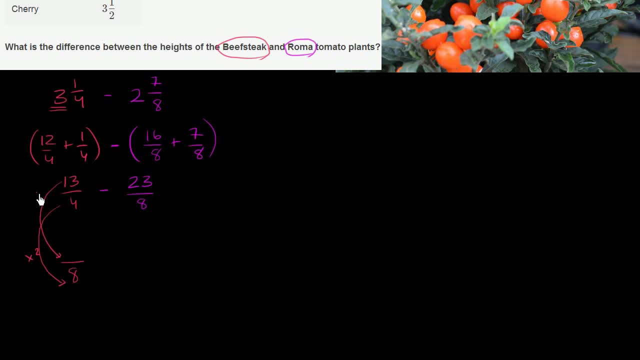 we have to multiply the numerator by that exact same value. We've got to multiply it by 2.. So this becomes 26 over 8.. And from 26 over 8, we're going to subtract 23 over 8.. And so this is going to be over 8,, 26 minus 23.. 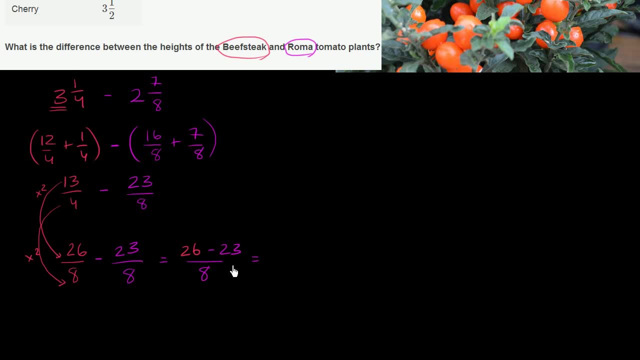 Minus 23,, which is equal to- and we deserve our drum roll. now, 26 minus 23 is 3.. So it's 3 eighths. So the difference between the heights of the beefsteak and Roma tomato plants: 3 eighths in everything. 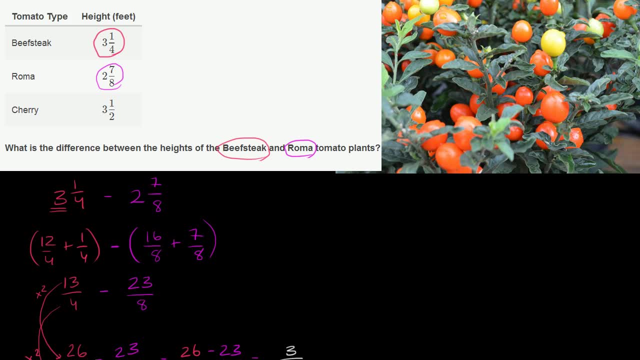 we've been doing in so far has been in feet, So 3 eighths of a foot.